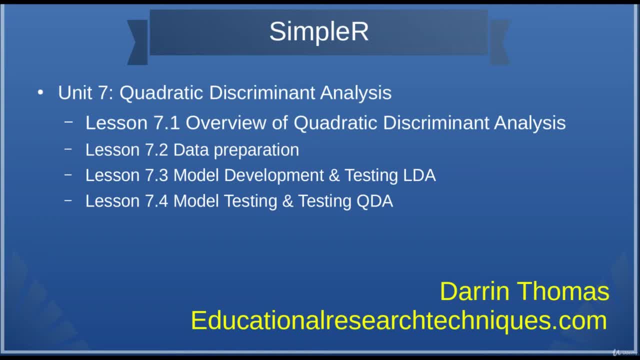 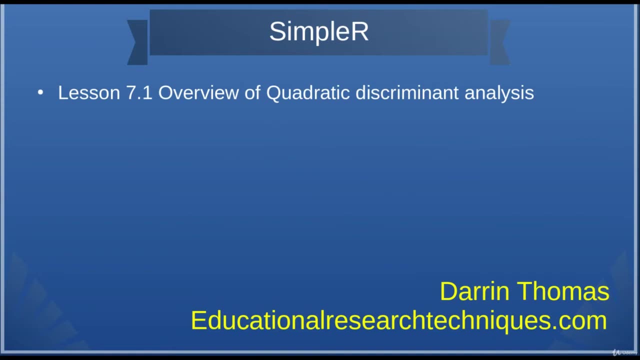 oh, there's a typo there. We'll be using model testing and we'll be using, basically using a quadratic discriminant analysis for the same data set, but this time, like I just mentioned, with quadratic discriminant analysis. So, having said that, I just want to give you a brief idea of the difference. 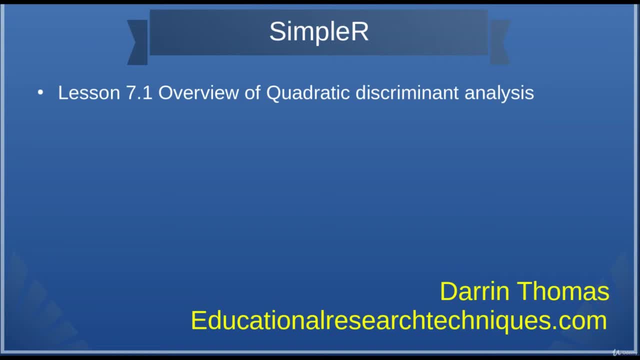 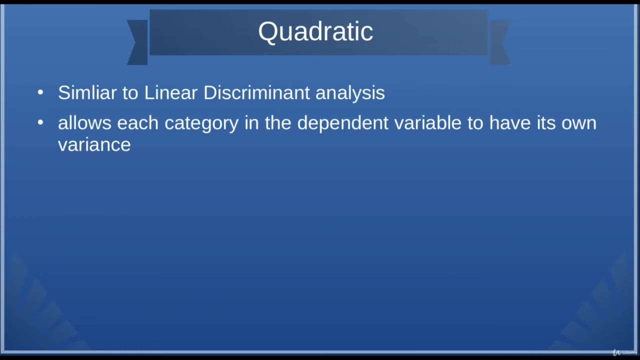 between linear discriminant analysis and quadratic discriminant analysis. It's not that shocking, but there are times when you might want to approach it from this angle, when you're trying to work with data rather than using just Regular linear discriminant analysis. So the primary difference is that with quadratic, 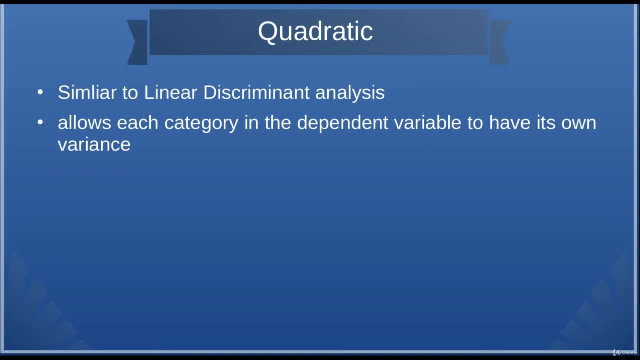 discriminant analysis, you are allowing each category inside the dependent variable to have its own variance. If you're familiar with t-test, you know that there are two types of t-test: one that is assuming equal variances between the groups and one that is not assuming. 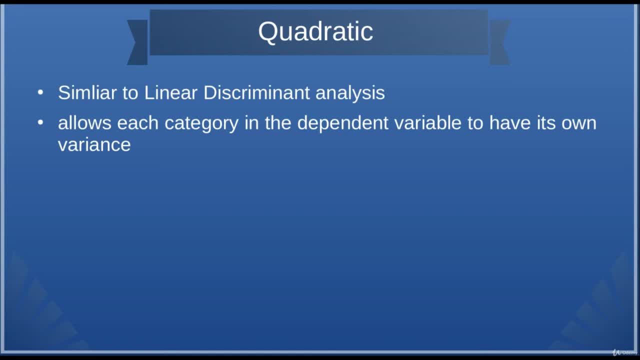 or that is assuming unequal variance between the groups. And so this is kind of the mathematical idea behind quadratic discriminant analysis, in that when you are using this particular algorithm, you are telling it that hey, you know the variances between the within the 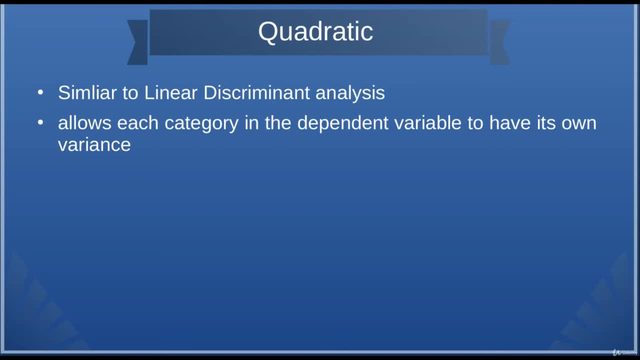 or between the groups is, for the groups is not the same. That's kind of what's happening, And now there's a whole lot that is happening mathematical behind, mathematically behind the scenes. but that is not the purpose of these videos. We're focusing on you learning. 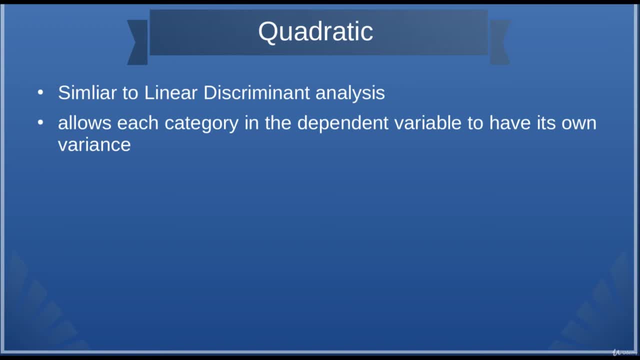 to apply the mechanics and use the mechanics of R to actually do things with data sets and to make Predictions and whatnot. but that's the main difference. Now, in terms of the similarities, again, you want to make sure that there's some sort of a clear separation between the. 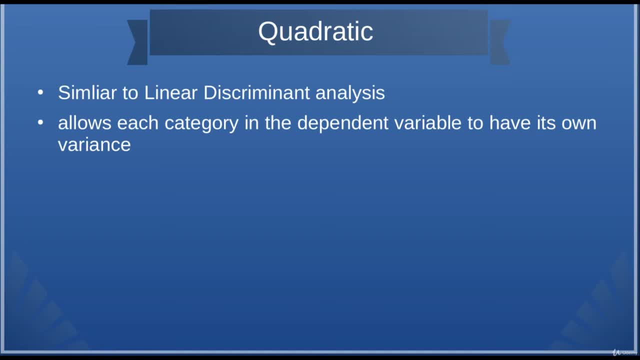 two groups- I'm sorry- Yeah, I'm correct- between the two groups that you're trying to predict, for if it's only two groups, If there's not a clear separation, quadratic discriminant analysis will struggle, just like linear discriminant analysis does, And we saw that in the prior. 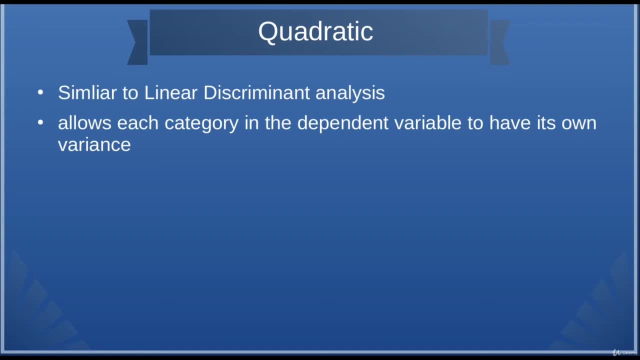 chapter. So that's the main thing. So now in the next video we're going to quickly go through our data preparation and we'll pretty much be ready to start developing our, our models for this chapter. So in this particular video, all we did was just kind of get an.